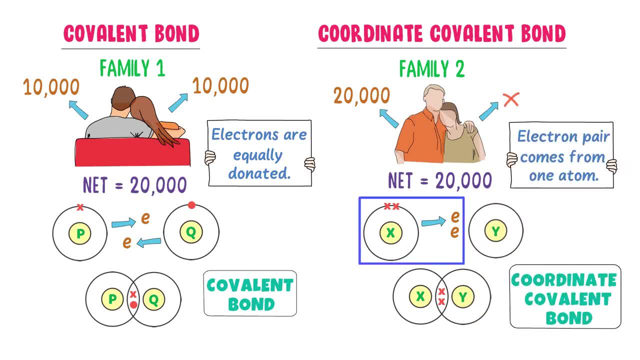 comes from one atom and the another atom just share that pair of electrons, While in the covalent bond the shared pair of electrons comes from both the atoms, from atom P and from atom Q. So this is the main difference between covalent. 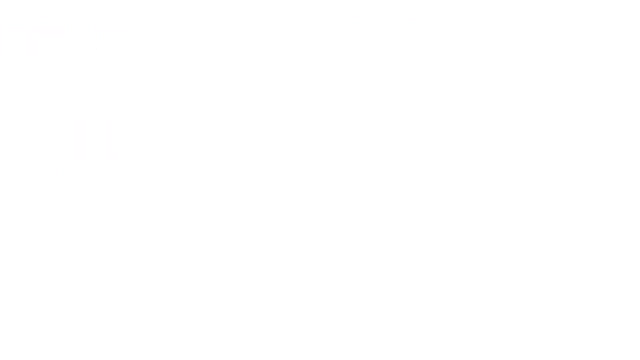 bond and coordinate-covalent bond. Now, what is coordinate-covalent bond? Well, we need lone pair and empty space in a valence shell for formation of coordinate-covalent bond. For example, consider oxygen atom and hydrogen atom. We know that there are six electrons present in the last shell of the oxygen atom. 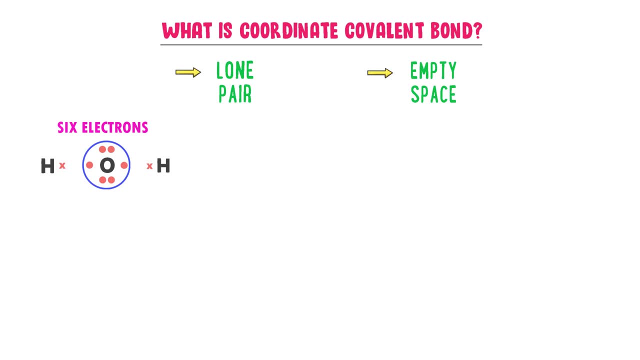 It needs more two electrons to satisfy its octet rule. On the other hand, in the last shell of hydrogen atom, there is only one electron. It needs only one electron to satisfy its doublet rule. Now hydrogen and oxygen will share one electron each to form a single. 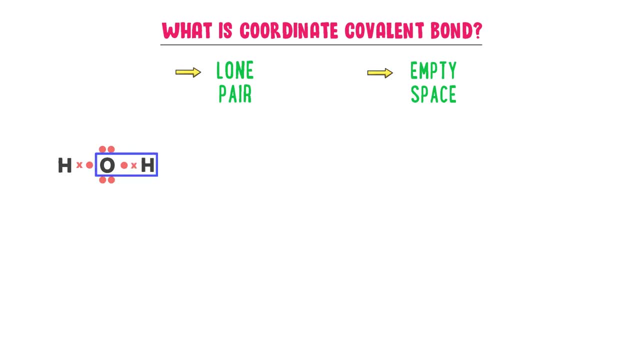 covalent bond. Another hydrogen atom will form a single covalent bond with oxygen by sharing one pair of electron. Now listen carefully. This pair of electron is called bond pair of electron. This pair of electron is called bond pair of electron. On the other hand, this pair 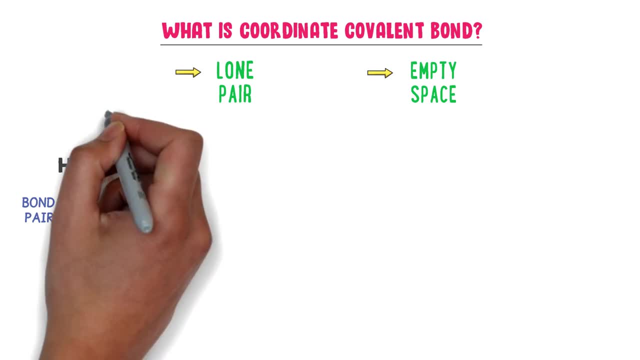 of electron is called lone pair of electron, and this pair of electron is also called lone pair of electron Because they do not participate in the covalent bond. they will not be able to participate in chemical bond. Now consider one another: hydrogen ion. The positive charge on hydrogen means that it 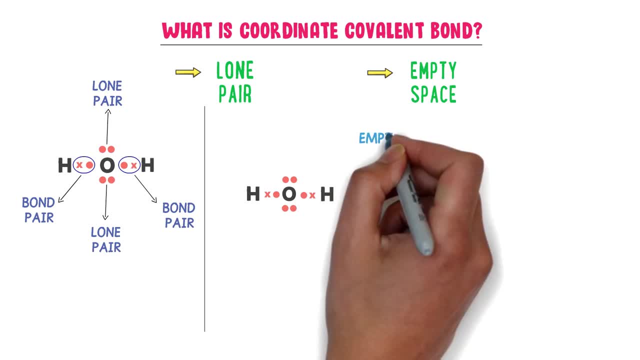 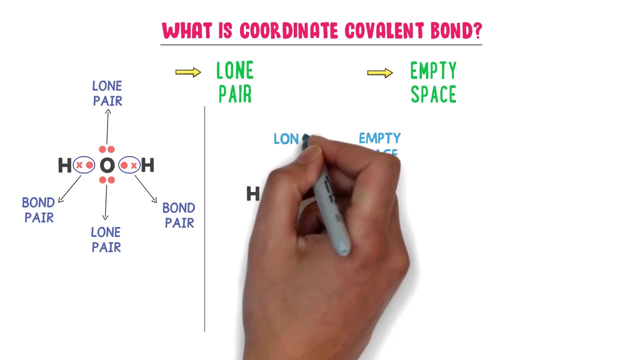 has lost one electron, So the valence shell is completely empty. It can easily accommodate two electrons Here. there is one lone pair with the water and there is empty space with the hydrogen ion, So coordinate-covalent bond will form between these two species. 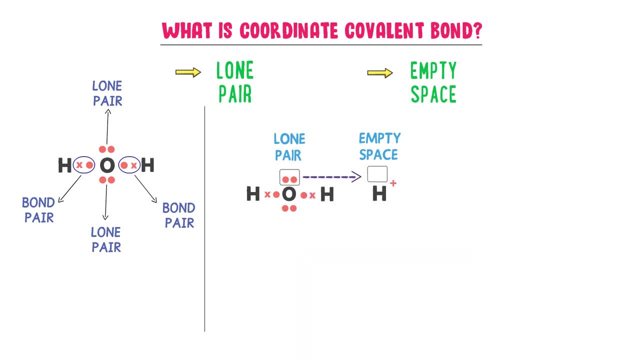 This lone pair of oxygen would be donated to this hydrogen ion. As a result of this, coordinate-covalent bond is formed and we get a hydronium ion Here. let me ask you What happens to these two donated electrons by oxygen. 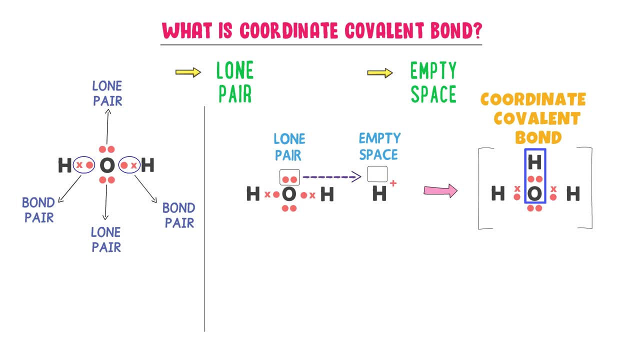 Well, these two electrons are shared by both oxygen atom and hydrogen atom. So the doublet rule of hydrogen is satisfied and the octet rule of oxygen is satisfied. Remember that this bond between oxygen and hydrogen is covalent bond. this bond between oxygen and hydrogen. 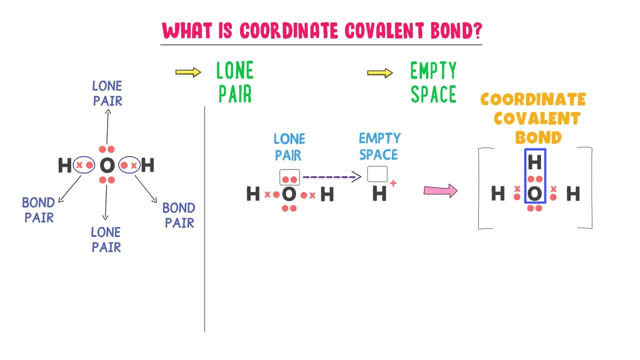 is also covalent bond, while this bond between oxygen and hydrogen is coordinate covalent bond. As a result of this, we get a hydronium ion and positive charge appears on it. This positive charge therefore appears on hydronium ion because water has gained proton, So we 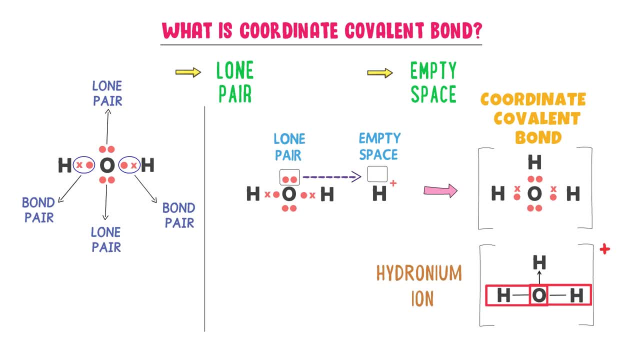 say that there are two covalent bonds present in hydronium ion and there is one coordinate covalent bond present in hydronium ion. Remember that this arrow represents coordinate covalent bond. So we say that the covalent bond in which only one atom donates the shared period. 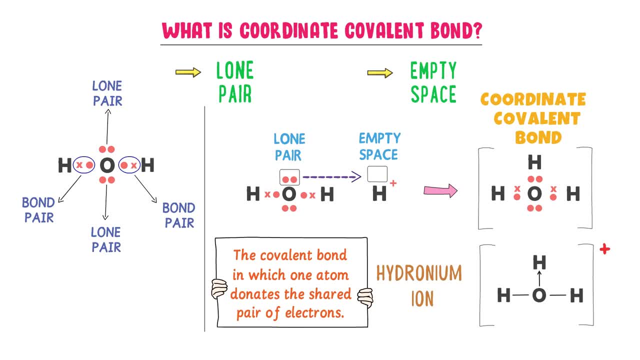 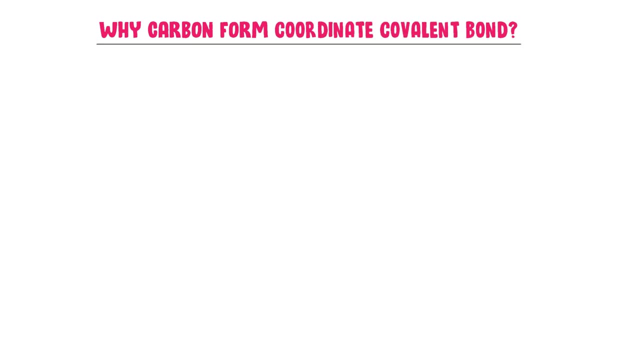 of electrons is positive. Now let me teach you one exam question. Why does carbon monoxide form a coordinate covalent bond? Well, consider carbon and oxygen. We know that in the valence shell of carbon there are four electrons, while in the valence shell of oxygen there are six electrons. 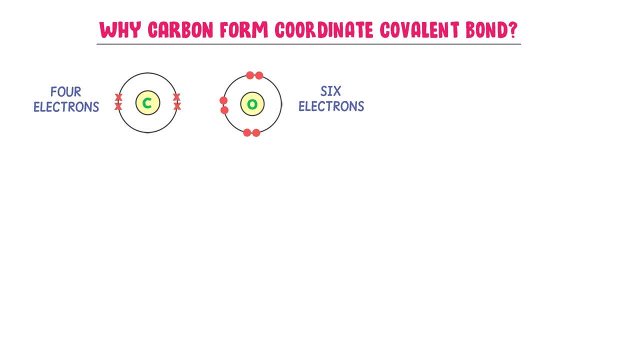 Carbon and oxygen share 2 electrons each to form double covalent bond and we get this molecule. We write C, double bond O. This is the double covalent bond, because we can see that two pairs of electrons are shared. Now let me count the total number of electrons. 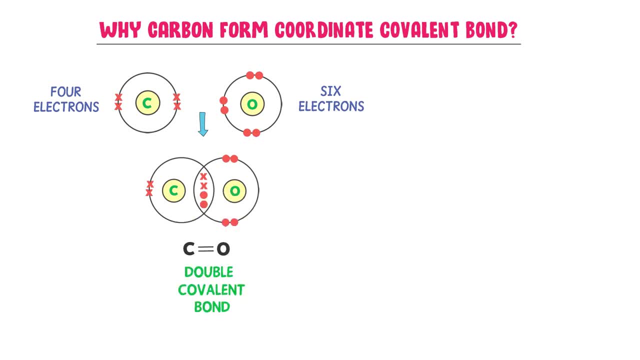 in the valence shell of oxygen: 1, 2, 3, 4, 5, 6, 7, 8.. There are 8 electrons present in the valence shell of oxygen. 2 electrons in chelonium are covalent bonds. This means that in the 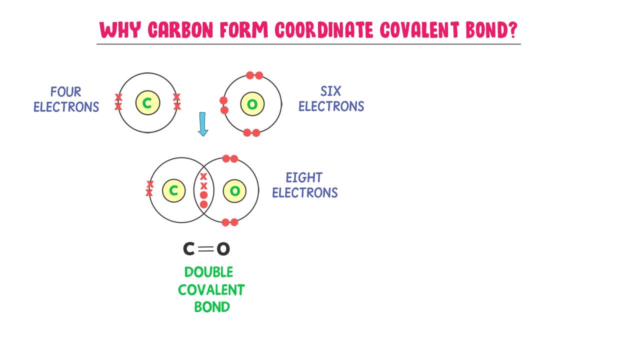 valence shell of student. that is ion, değer 0.5 electron of electrons present there, value $不是8. This and o$0. Maintenant, we get that here. choppeduko qualities oxygen atom, So its octet rule is completed and it is a stable atom. Secondly, let me count the.